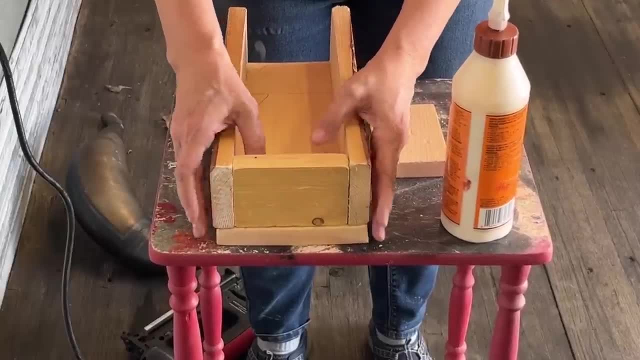 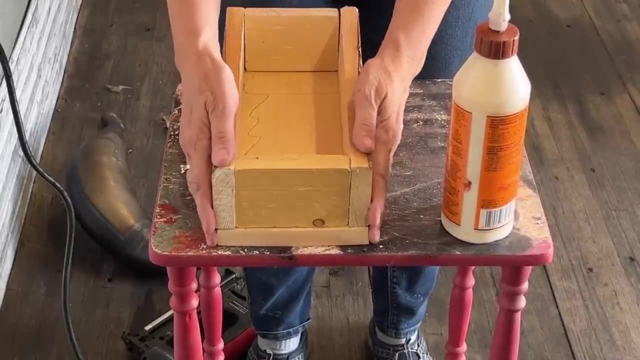 your starts by ensuring all the pieces fit along the showing that you want, and all the pieces have 화 the base. i've cut all the wood using my chop saw, which i actually found at a pawn shop. this is the best place to find tools at a fraction of the cost and they'll still be really good quality and i 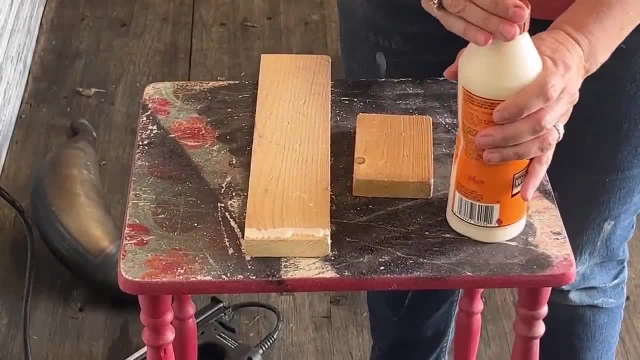 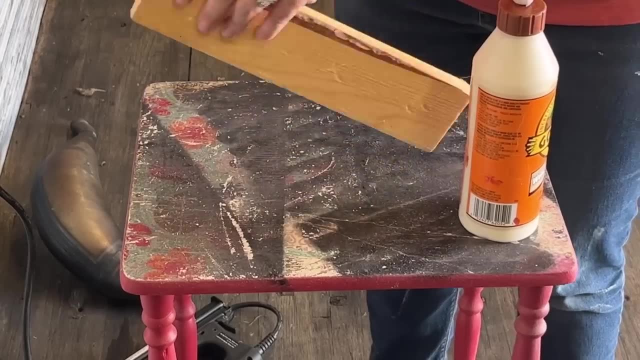 also found this brad nailer for just 30. it works like a charm, but don't worry if you don't have one. you can always use screws, or you can opt for the classic hammer and nails to put this piece together. there are plenty of options to choose from, so just go with what works for you and the 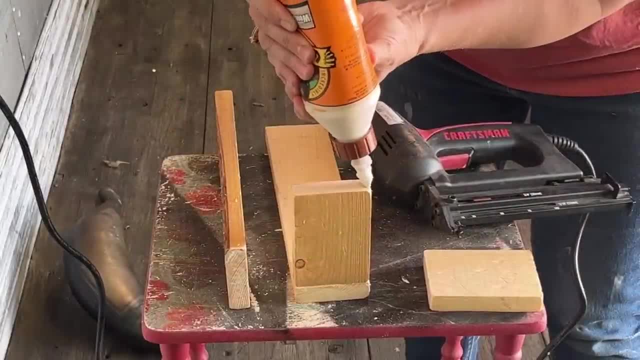 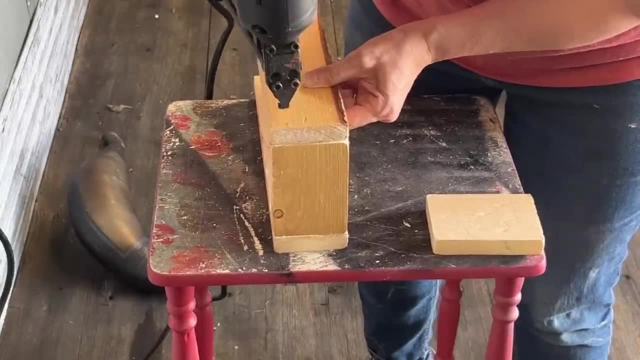 tools that you have to secure all these pieces. i'll apply a small amount of wood glue and then i'm going to use my brad nailer to secure them in place. once that's done, we'll be ready to attach the base. if you're interested in earning some extra cash with diy projects, the ones 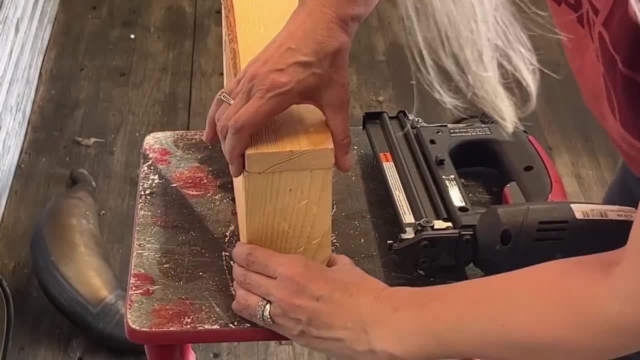 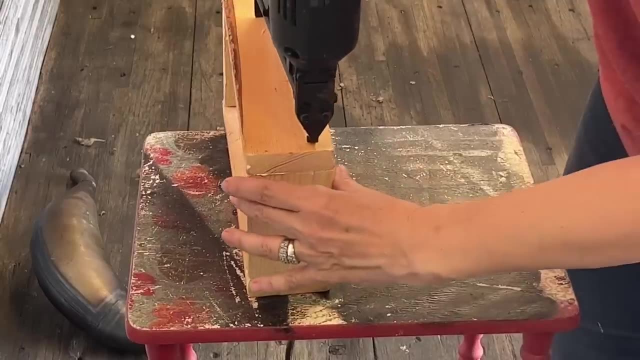 featured in this video are a fantastic starting point. they're incredibly simple to assemble and they won't break the bank, especially if you can find free wood. also, these projects happen to be among my top sellers. the best part is, you don't need an extensive collection of 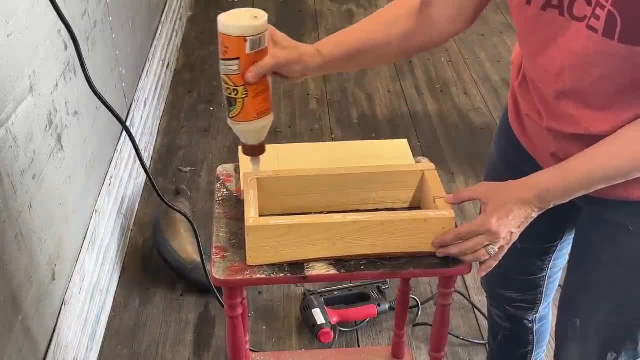 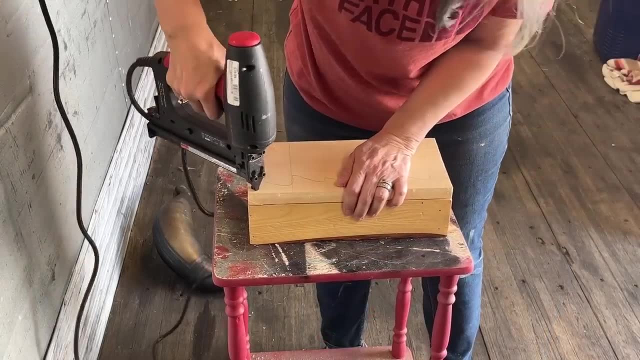 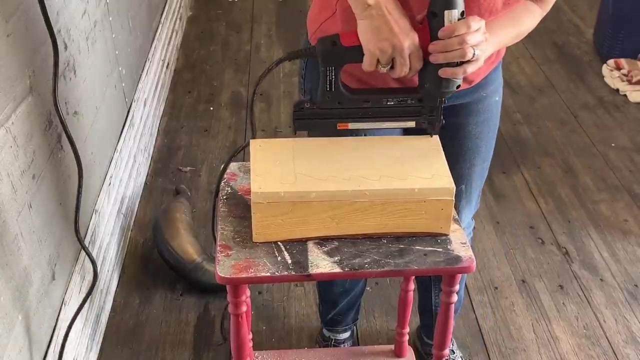 tools or special products to complete them. plus, they offer endless possibilities for customizing. you have so many choices when it comes to finishing these projects. you can leave them just the plain wood, you can paint them in vibrant colors or you can even add graphics. the possibilities truly are endless. find out what's selling best in your local market. 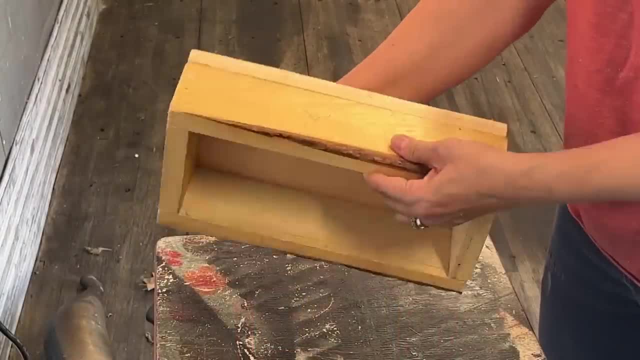 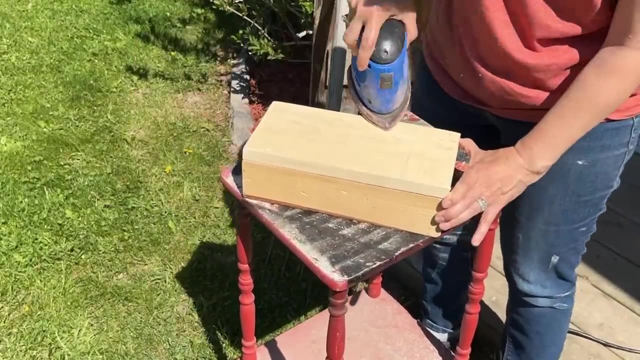 in my experience i've found that that rustic charm of the plain wood is selling really well right now. after putting the box all together, the next step is to give it a really good sanding with some 80 grit sandpaper. now comes the exciting part: staining. i highly recommend. 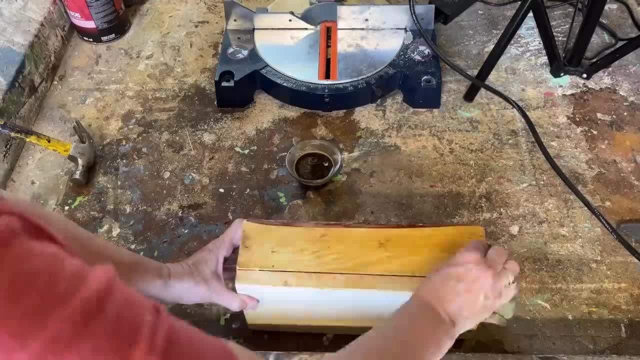 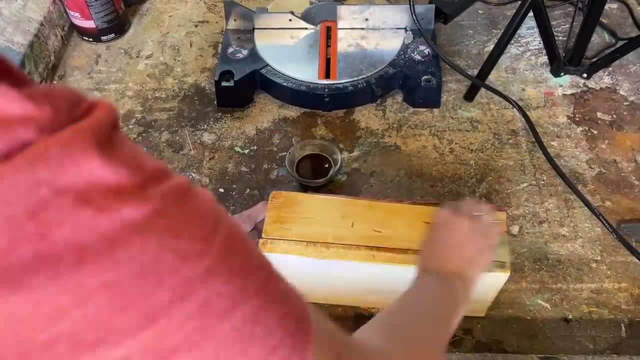 trying out a budget friendly and fantastic alternative called coffee staining. trust me, it works wonders. all you need is some instant coffee and some hot water. simply rub that mixture onto the wood and you're going to see the grains come alive with beautiful color. it's an affordable 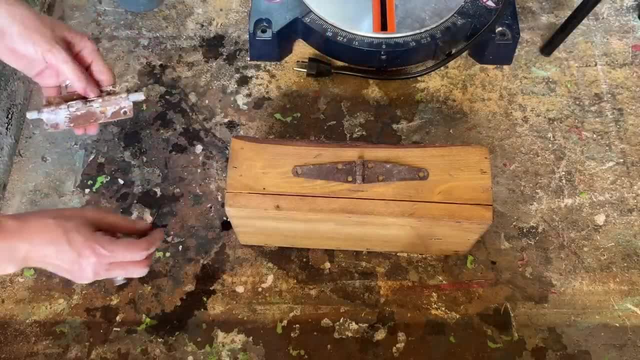 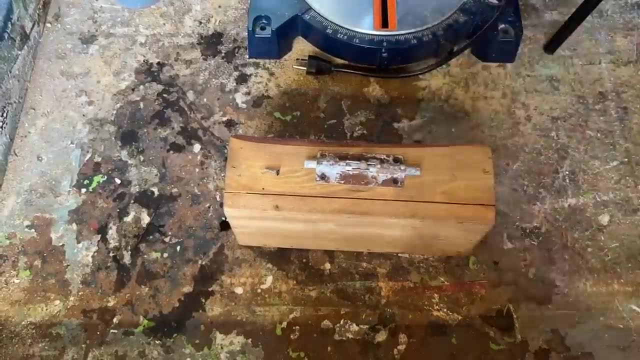 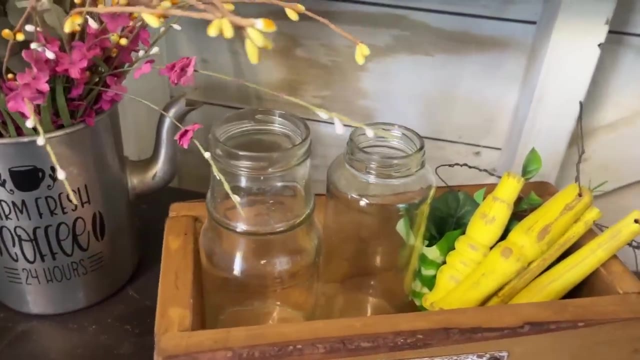 option that provides stunning results. this is going to save you from having to purchase expensive stains. give it a try and you'll be amazed at how well it works. to complete the box, i wanted to add a hardware detail on the front. luckily, i found a rusty latch in my stash and i attached it to the box using some screws. it gave a nice 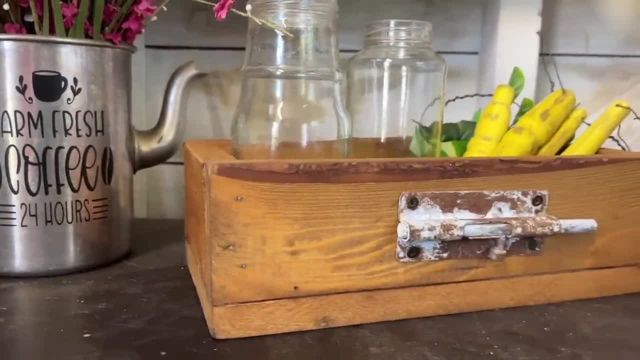 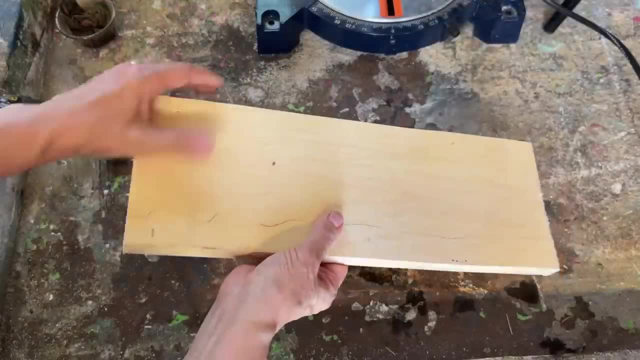 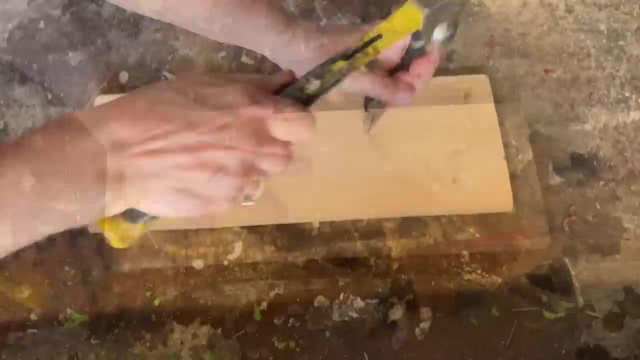 finishing touch. this is such a simple diy project and it's a great way to make some extra cash to sell them, so try this out. this diy project is incredibly simple and so easy to do. all you need is a scrap piece of wood, a hammer, a chisel, a pair of pliers, some nails and we're going to create that old, rustic look putting. 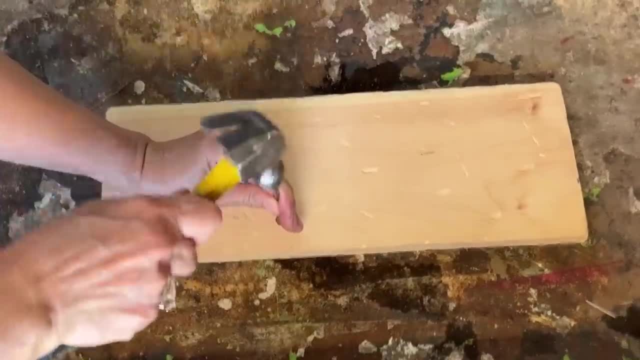 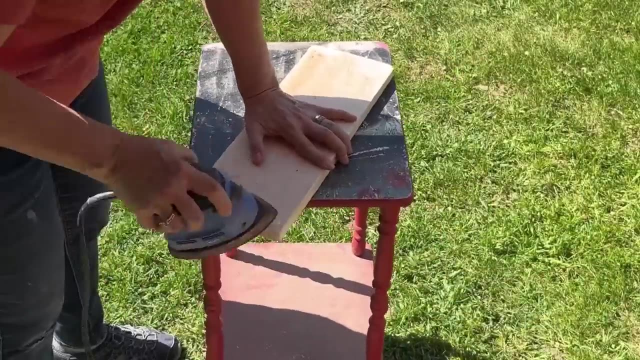 dents in it, weathered holes and before moving on i'm going to take it outside and give it a sanding with some 80 grit sandpaper, just to soften it up around the edges. for staining i found a great deal at our local hardware store: a two dollar mistin in a really beautiful color. i'm 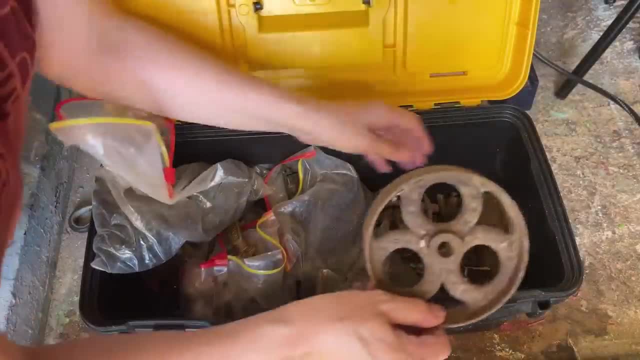 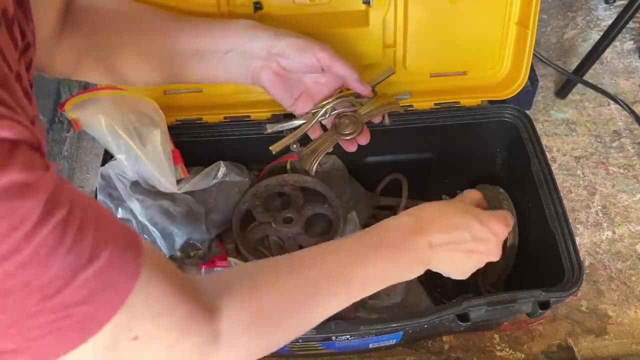 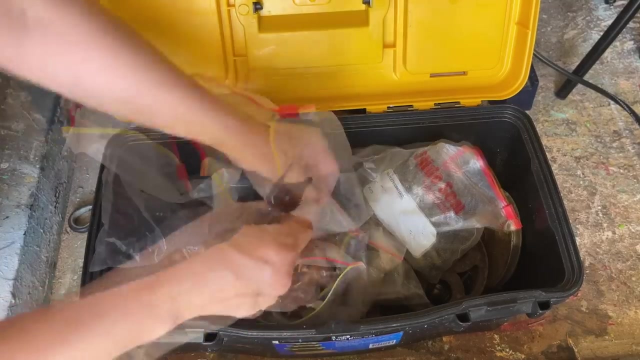 going to apply that stain on the wood and it looks fantastic. now onto my stash of hardware. i keep a toolbox filled with full of various handles and knobs and pulls that i can browse through when i want to find something that's going to be a perfect fit. i think these pulls will work perfectly. i also have a container. 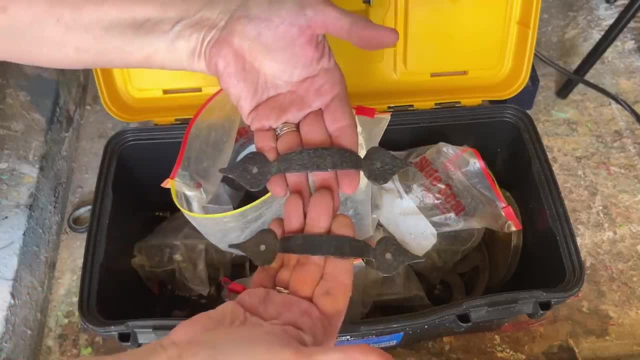 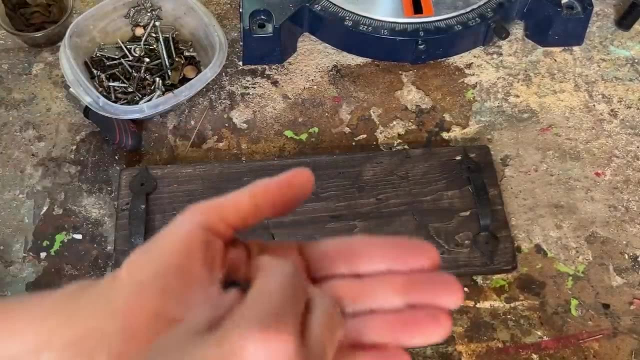 filled with nails and screws that i know come in handy for these type of projects. i'm going to simply screw these two handles onto that piece of wood and that's it. it's that easy. to finish it off and protect the wood, i'm sealing it with some poly acrylic sealer. this diy is so versatile. they make 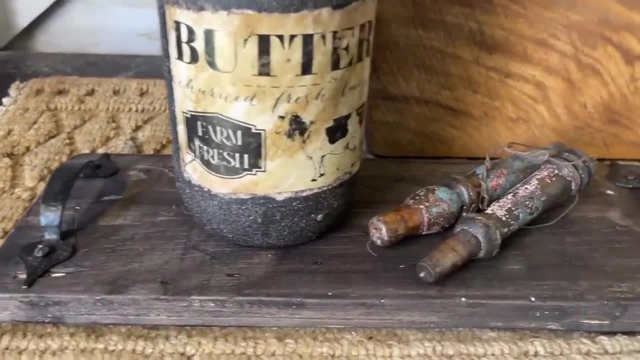 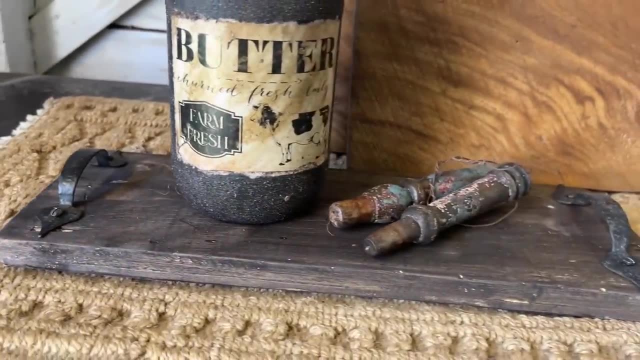 a great addition to a kitchen for holding your kitchen, kitchen, kitchen, kitchen, kitchen kitchen scrubbers or dish soap, or you can put them out on your dining room table or out in the patio. it's an effortless diy that's both functional and has a lot of charm. another diy project that can help. 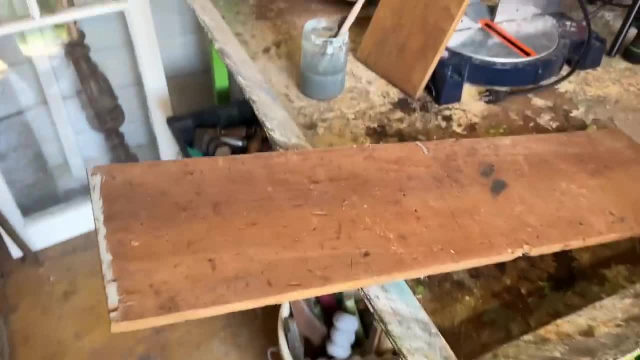 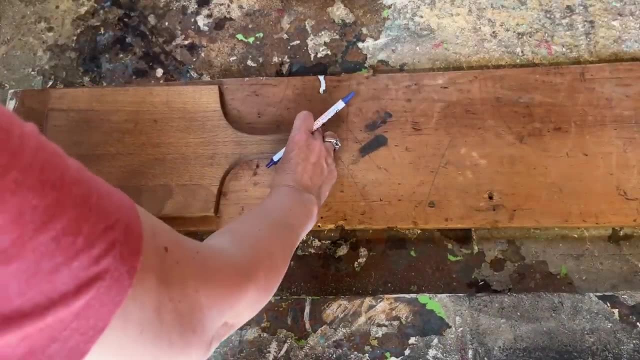 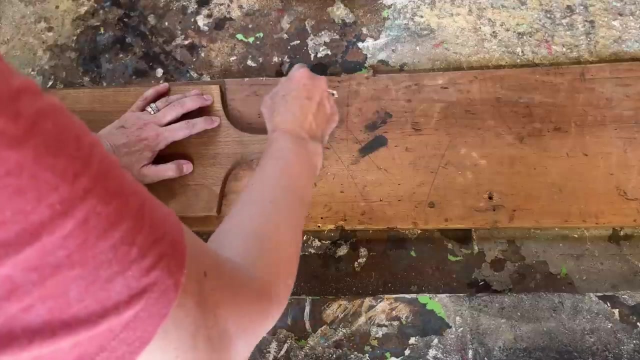 you earn extra cash is making breadboards. these have been incredibly popular for years and the best part is they're super easy to make. i have a breadboard that i keep in my craft room and it serves as a handy template. now i have this scrap piece of wood that's full of character. it has 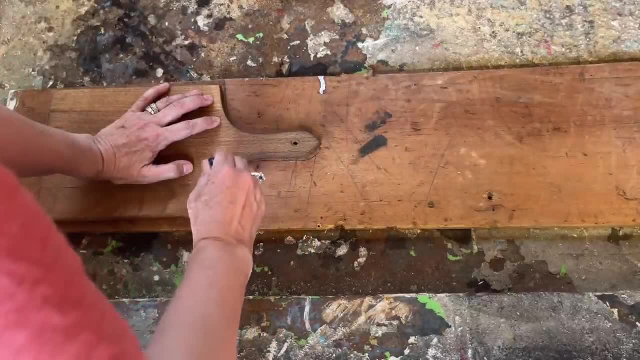 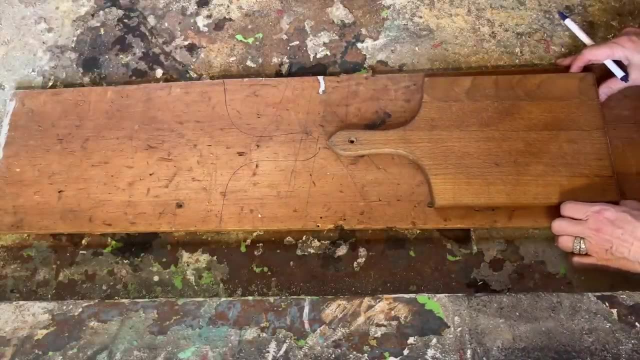 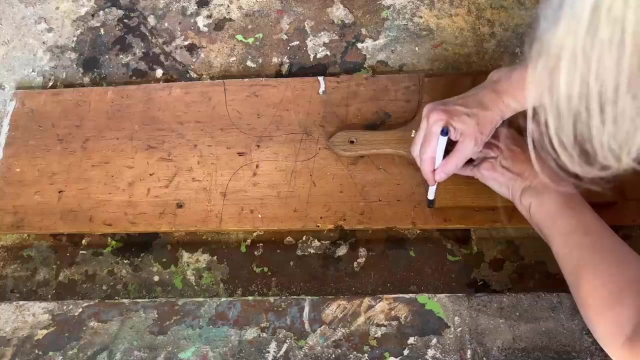 a little bit of a mix and dings and it has that aged look already. i'm simply going to trace the shape of the cutting board onto it. i can get two cutting boards out of this one piece of wood, making it a really profitable diy. i'm going to take it outside and i'm going to use my jigsaw. 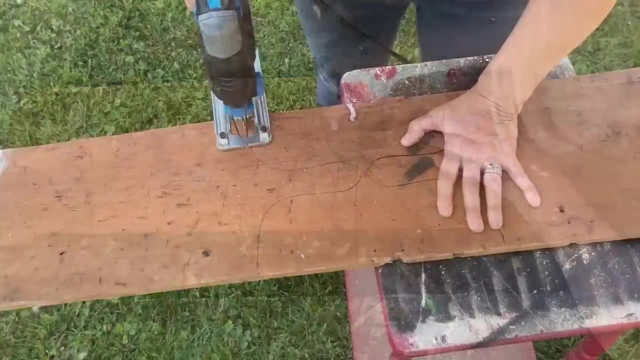 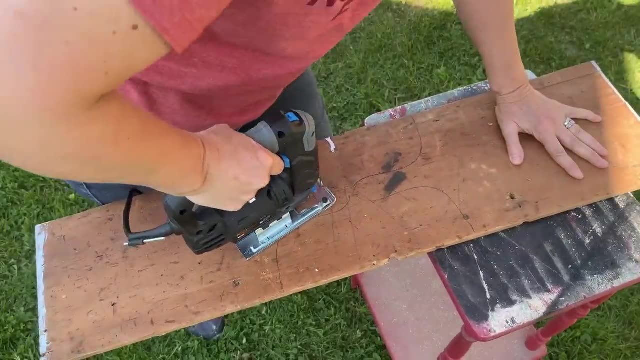 and carefully cut out the shapes. don't worry about feeling intimidated by jigsaw. they're actually quite easy to use and if you don't have one already, i recommend checking out your local pawn shop for some great deals. you might be surprised at how affordable they can be, but they're. 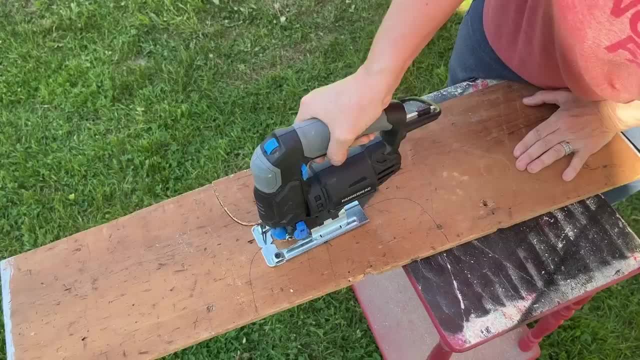 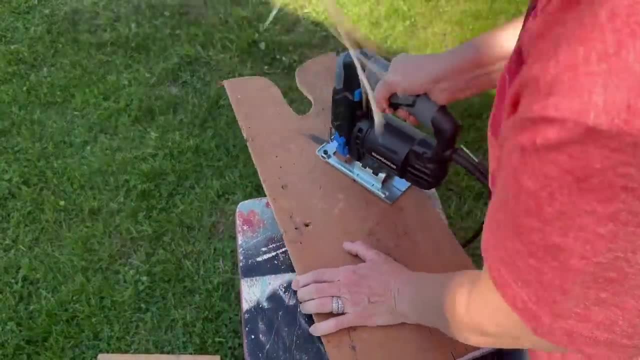 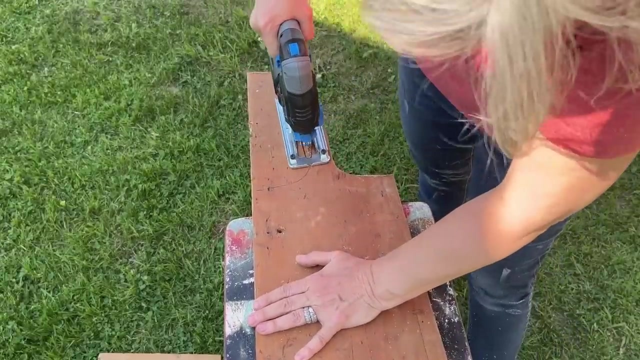 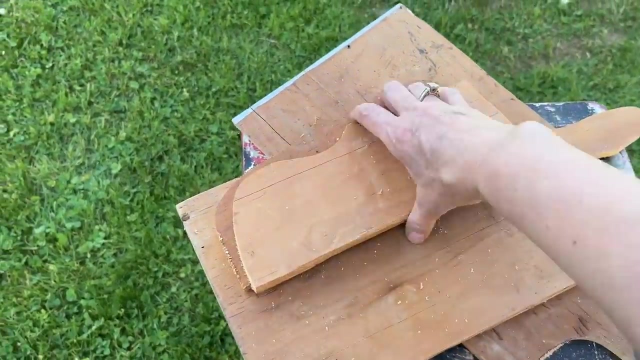 you can also find brand new ones really reasonably priced on amazon. i'll provide that link down below in the description, now that i've finished cutting them out. remember not to throw those leftover pieces. we can use them for another diy project later on. i'll stash them away. for now, 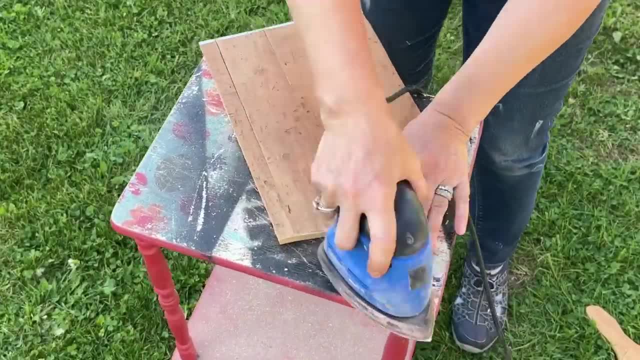 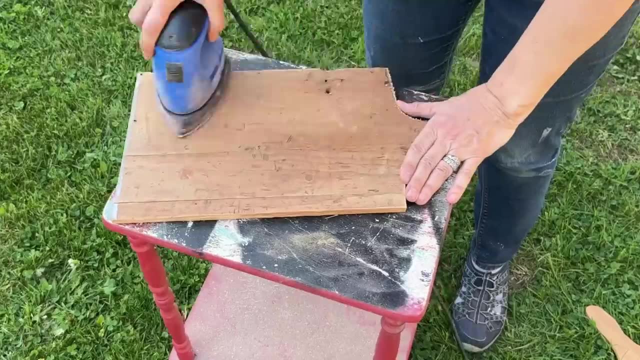 next, i'll take these red boards outside and i'll use some 80 grit sandpaper to give them a smooth, polished finish. these boards already have so much character, so i don't want to sand them too much. i want to preserve that charming, worn out look. most of these bread boards are primarily 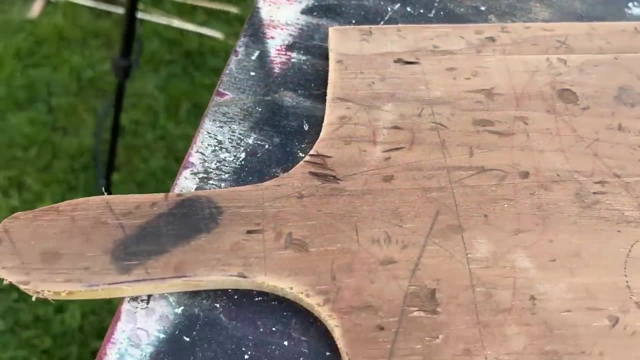 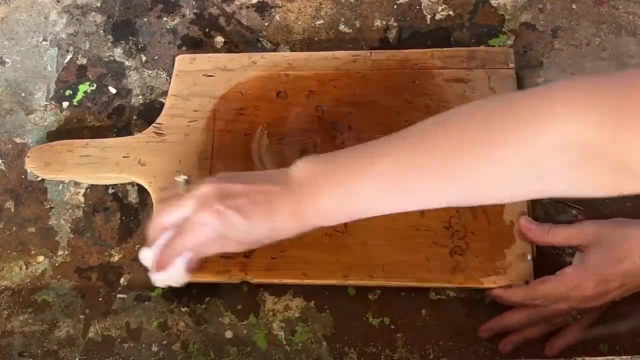 intended for decorative purposes. however, if you happen to be working with brand new wood and you know its type, i encourage you to do some research. find out how you can make these boards food grade and suitable for use in the kitchen. it's important to ensure that they meet the 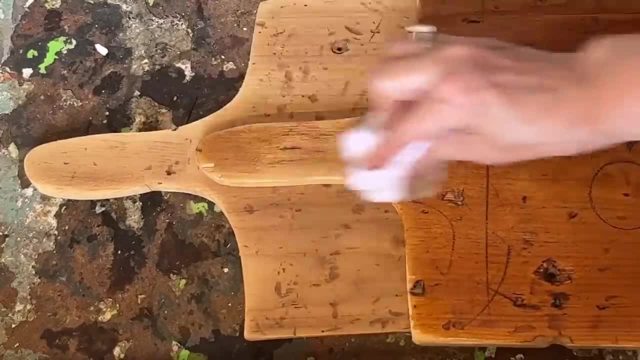 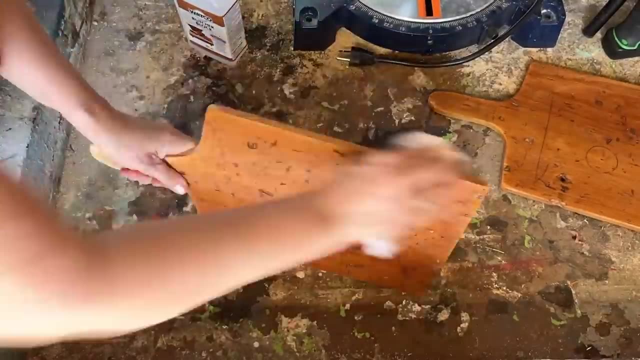 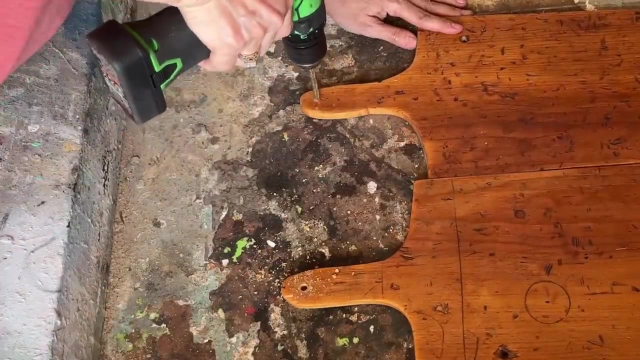 necessary standards and are safe for food preparation. to enhance the beauty of these boards, i've decided to use some leftover butcher block from a previous project. i'm applying this oil and it really highlights the gorgeous grain of this wood and the end result is simply stunning. for the finishing touch, i'm going to drill a hole in the top, add some twine. one of the breadboards 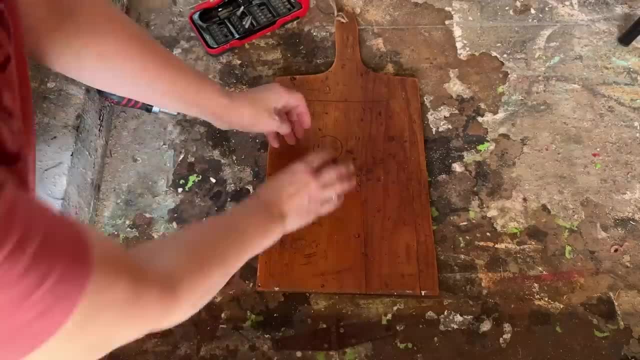 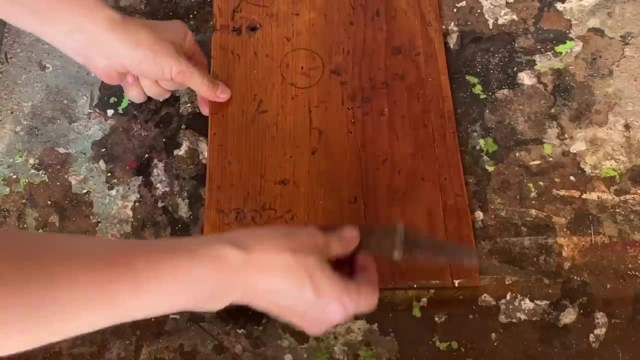 had a crack at the bottom, so i came up with a clever solution to prevent further cracking. i found an old, rusty hinge in my stash, along with some matching screws. i'm going to attach that hinge right between the crack and the wood. This addition should not only reinforce the board. 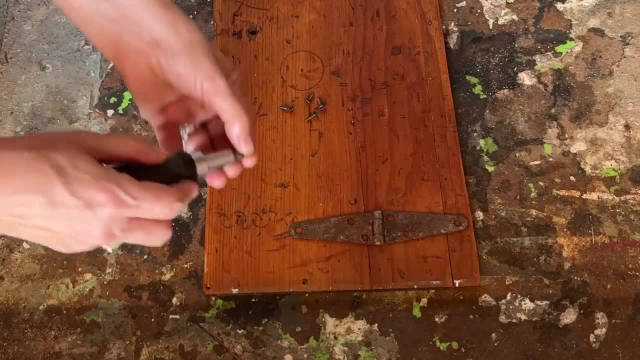 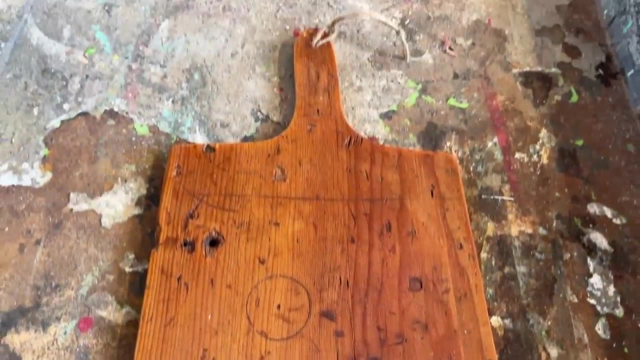 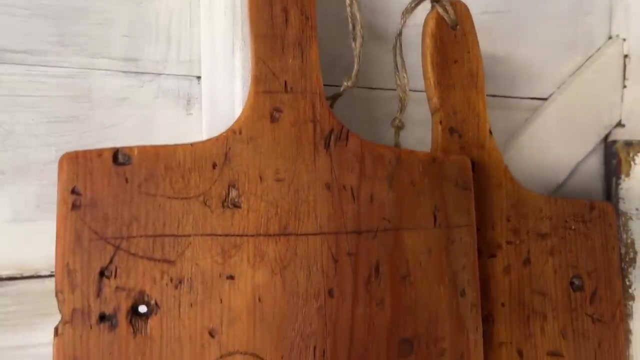 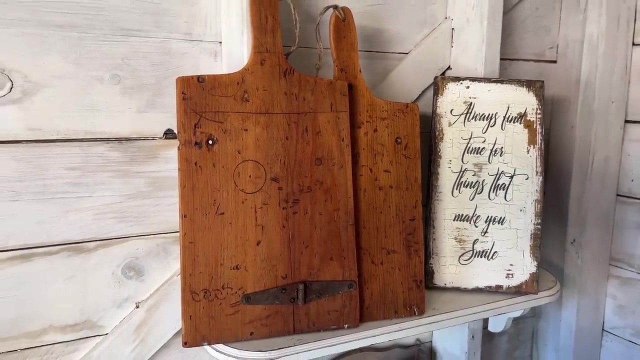 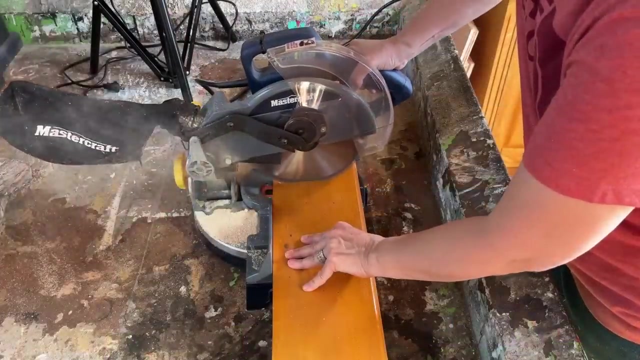 but it's also giving it a charming farmhouse feel. It's these unique touches that make each board one of a kind, and it also helps them sell better- Another best-selling DIY, and I love making these, And the best part is they're incredibly easy to assemble. 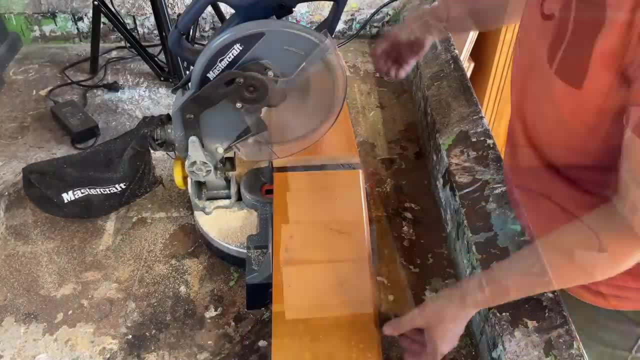 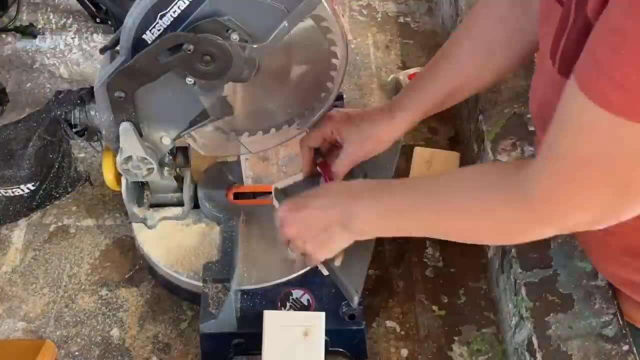 just using scrap wood For this project. I used an old piece of wood that I believe was part of an old dresser, along with some leftover ends of two-by-fours. With these materials, we're gonna put everything together and create a fantastic riser. 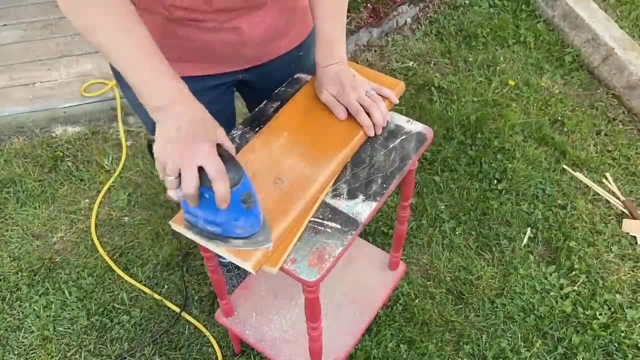 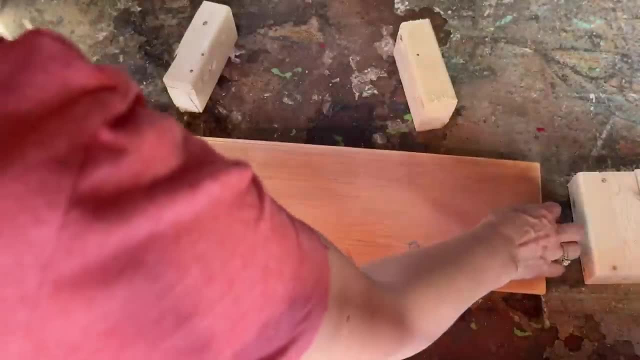 I've got enough material to make two risers, so I'm gonna cut the two-by-fours so they're all the same length. I'm gonna sand down that scrap piece of wood that I've cut in half, and then we're gonna put it all together. 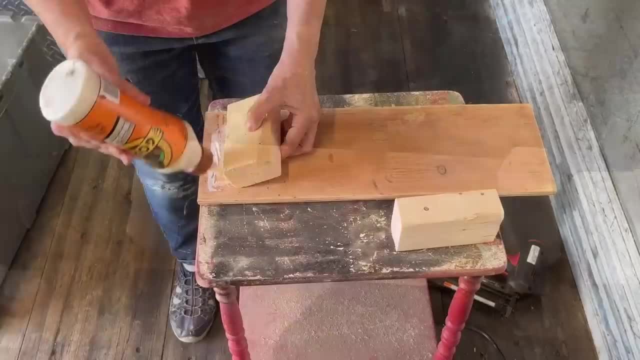 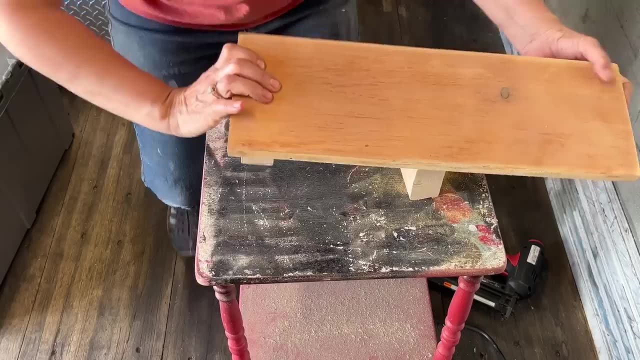 Two-by-fours will serve as an adorable feet on the riser. If you're feeling creative, you can also use spindles or even caster wheels to add a unique touch. Once assembled, these risers become one of my top-selling items. 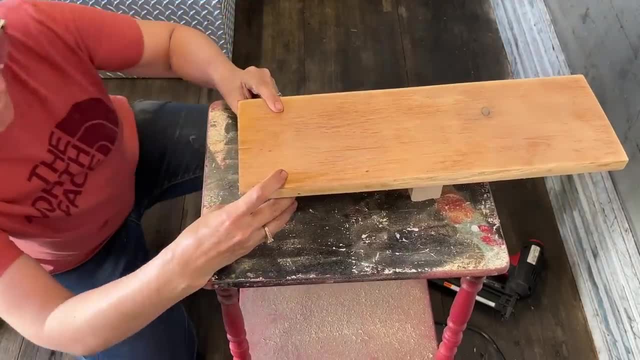 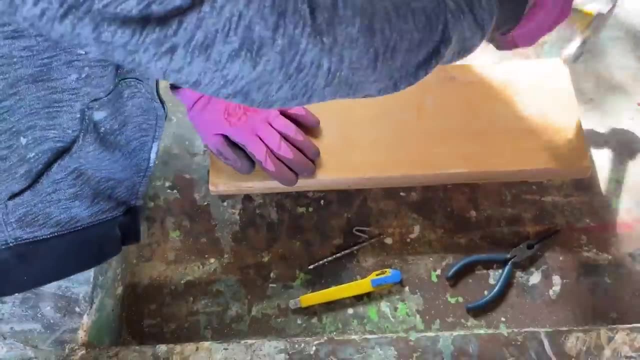 To ensure the perfect placement, I'm gonna center that two-by-four underneath the wood and then I'm going to use my brad nailer and put it all together. I also added a little bit of wood glue, also To ensure the perfect placement. 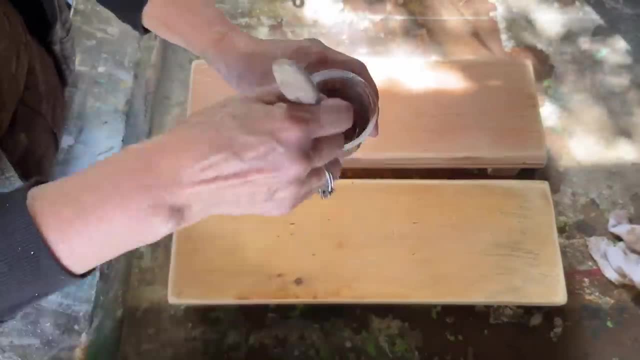 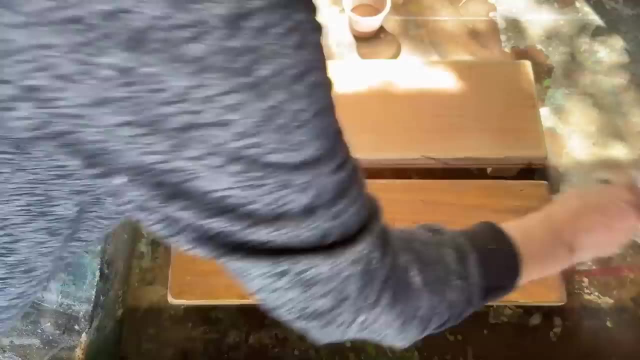 I'm gonna center those two-by-fours underneath the wood, adding a little bit of wood glue and then brad nailing it into place. Now I've mixed up some DIY stain. This is really popular right now and it gives that rustic, weathered look. 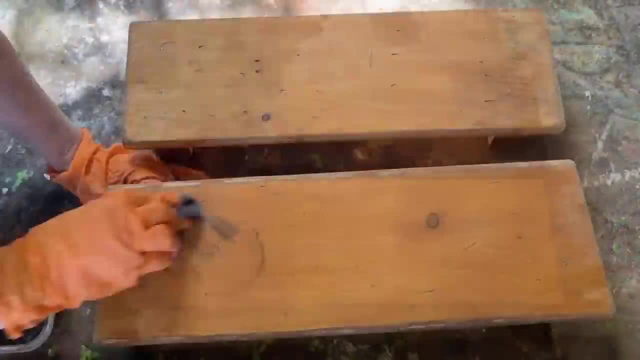 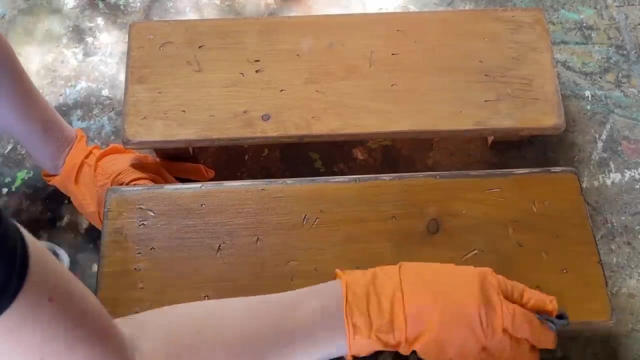 that complements that farmhouse or primitive style that everybody wants. right now I have a full tutorial on how to make my DIY stain. I'll put the link to that down below in the description. And to finish it off, I'm adding some dark antiquing wax. 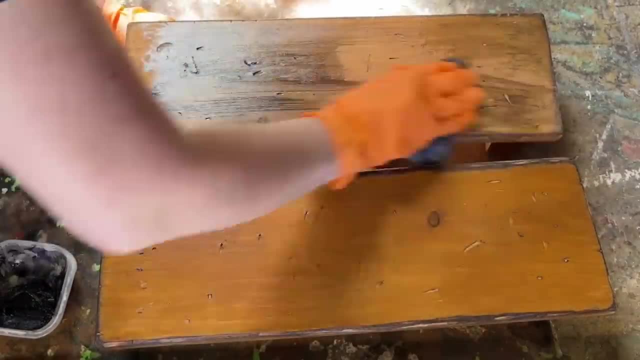 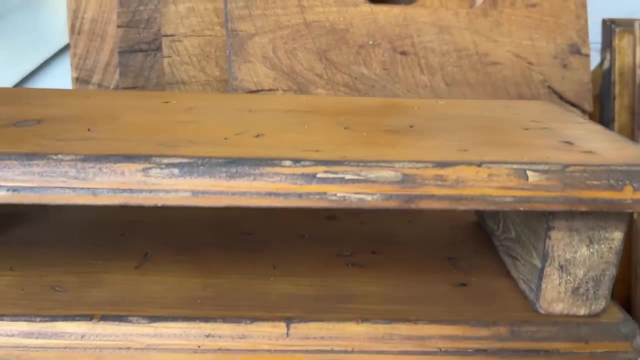 It's just going to fill up those little nooks and crannies and give it a really aged look. that I'm trying to accomplish. And now I've completed two risers that I know are gonna sell super fast, And if you wanna know how to price your DIYs, 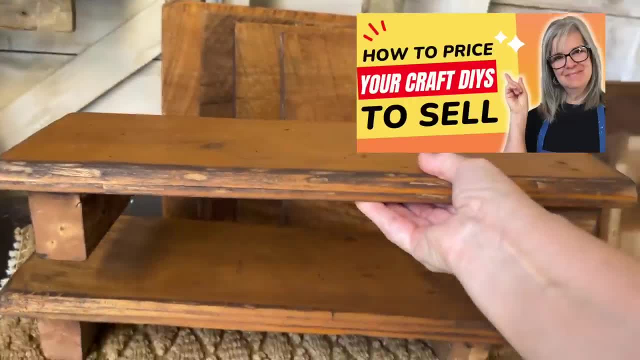 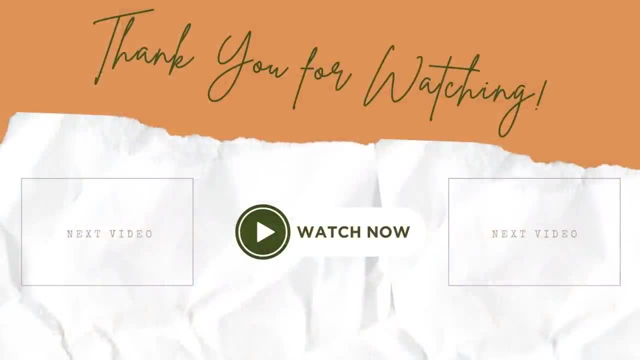 I have a full tutorial on the formula that I use. I'll put the link to that down below in the description and you can watch that after this video. I hope these DIY projects have sparked some inspiration. Let me know down in the comments which one was your favorite. 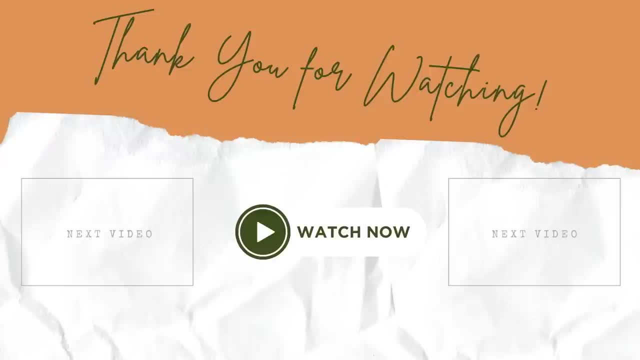 Thanks for watching, Have a great day and we'll see you in the next video. 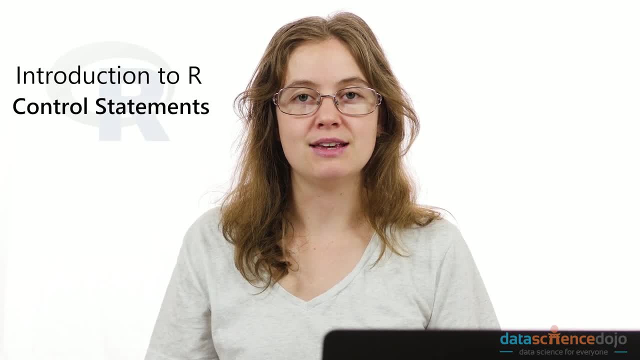 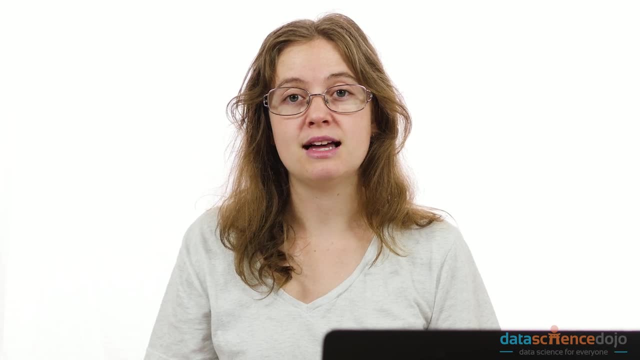 Let's just say you need to check through a column vector of data values to see if it meets a certain condition, or only execute a function if it meets a certain condition. In this example, we need control statements that allow us to control the flow of a program. There are quite a few control statements.